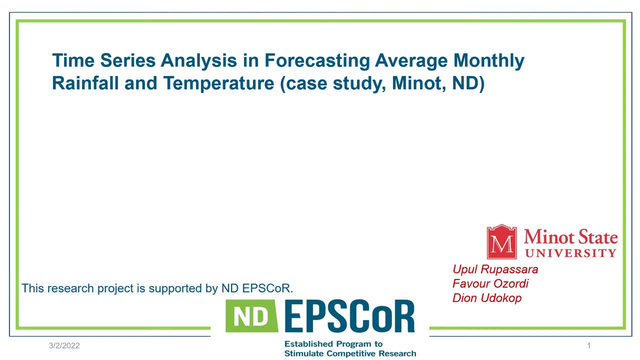 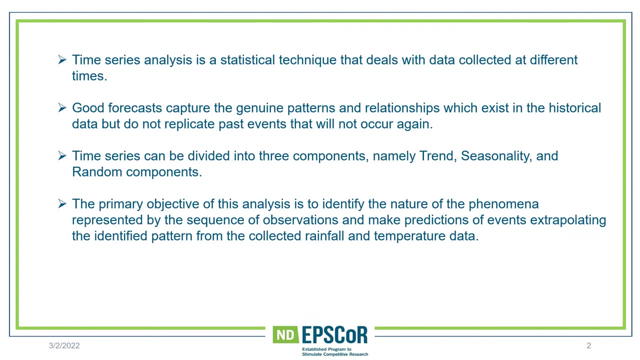 Time series analysis in forecasting average monthly rainfall and temperature. This is the case study based on Minot, North Dakota. This research project is supported by North Dakota established program to stimulate competitive research. Time series analysis is a statistical technique that deals with data collected at different times. Time series can be divided into three major components: trend, seasonality and random components. 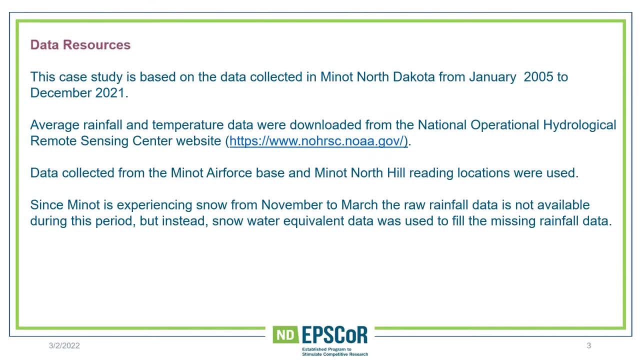 Average rainfall and temperature data were downloaded from the National Operation Hydrological Remotions Institute website. Since Minot is experiencing snow from November to March, the raw rainfall data is not available during this period, But to institute snow water equivalent data was used to fill the missing rainfall data. 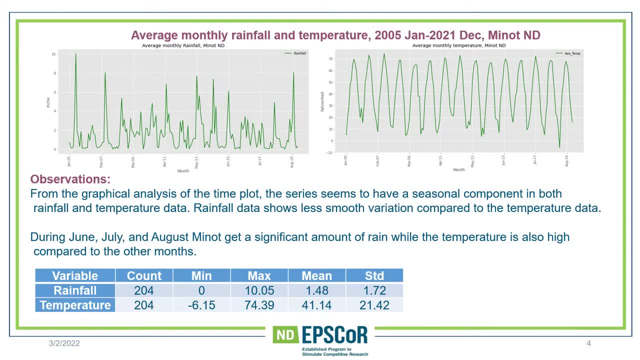 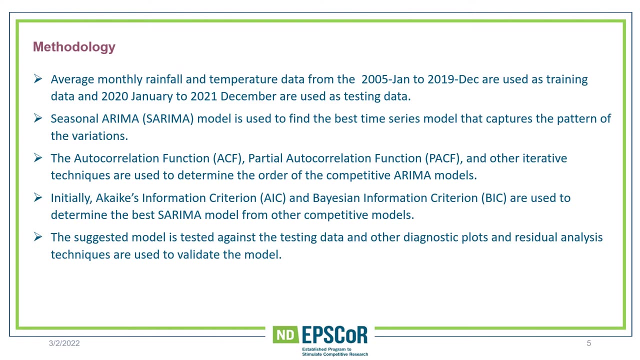 These two figures shows the time series for rainfall and temperature data. Also, the table shows the basic data And the table shows the basic descriptive statistics for both time series. The methodology: Since we could see there is a seasonal component, we use seasonal arima model. 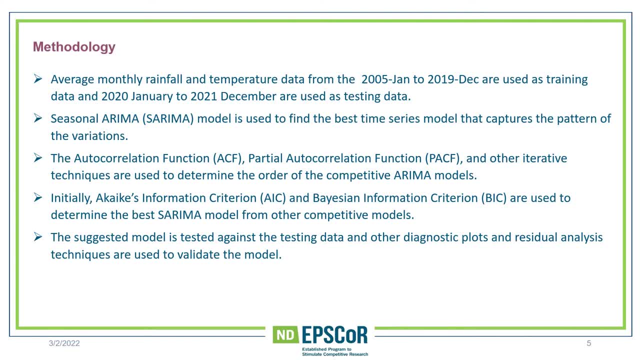 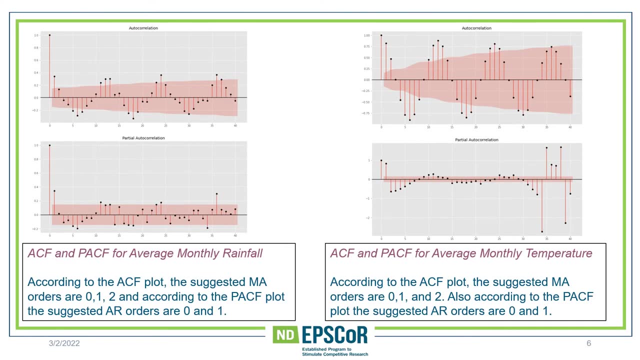 The ACF and PACF were used to determine the order of AR and MA component. Also the Akaike Information Criterion and the Bayesian Information Criterion is used to determine the best arima model from the competitive models. Those are the ACF and PACF plots for both rainfall and temperature. 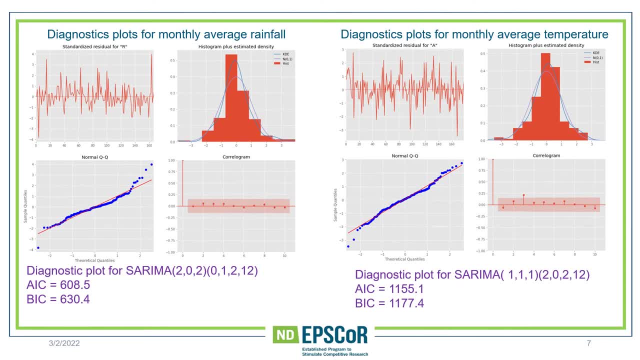 Those two plots shows the diagnostic plots for rainfall and temperature data. We could found that the best arima model that can be used to forecast the rainfall is 202012.. These two will represent the seasonal component. Also, the best model for the temperature data is 111202. 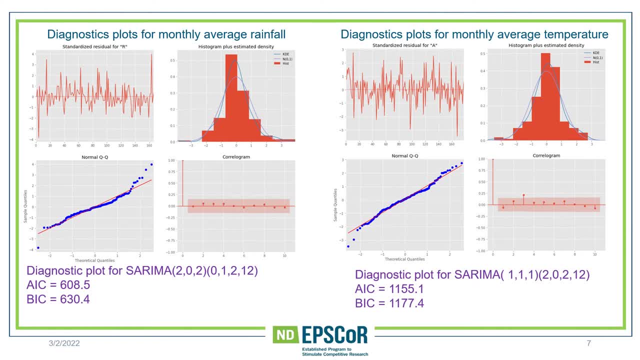 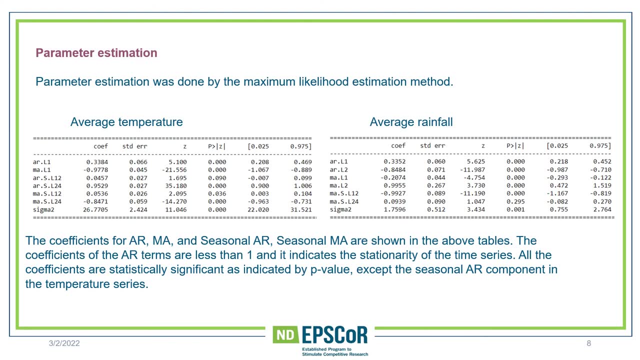 Also those are the models that we found to have the lowest AIC and BIC. So those are the parameter estimations for both rainfall and temperature. So we can see all the coefficients are significant because they have very small p-value. 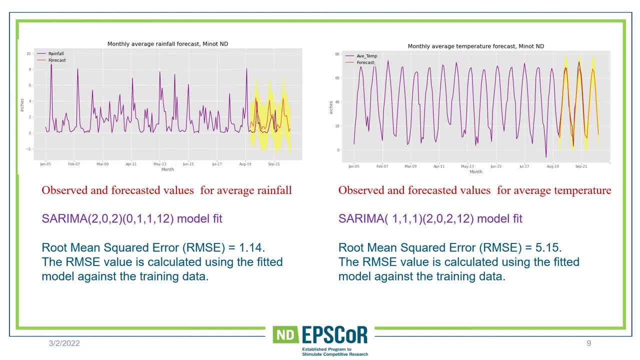 These two figures shows the observed and forecasted values for average rainfall and also the temperature data. So the root mean square error for rainfall data is 1.14.. Also, the root mean square error for temperature data is 5.15.. 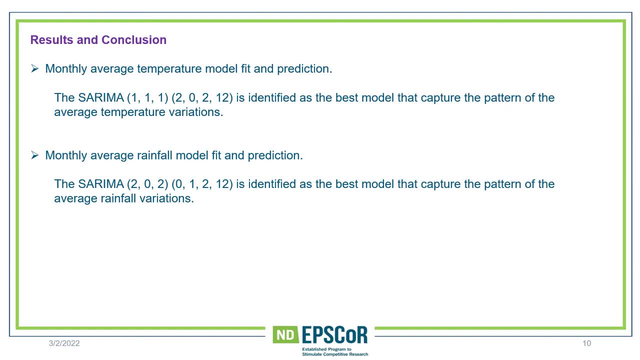 The SARIMA 111202 is identified as the best model that capture the pattern of the average temperature variation. Also, the SARIMA 202012 is identified as the best model that capture the pattern of the average rainfall variation. Thank you,